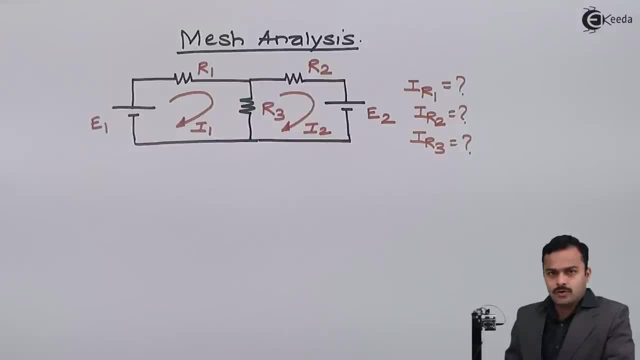 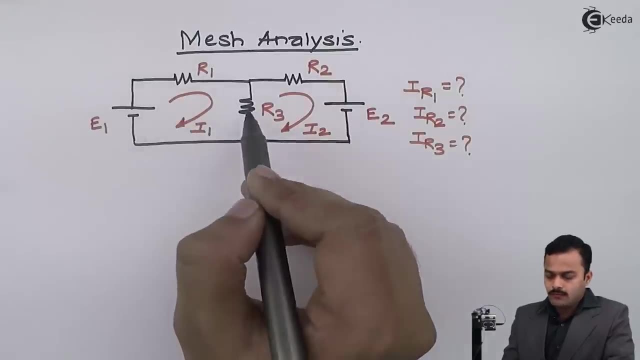 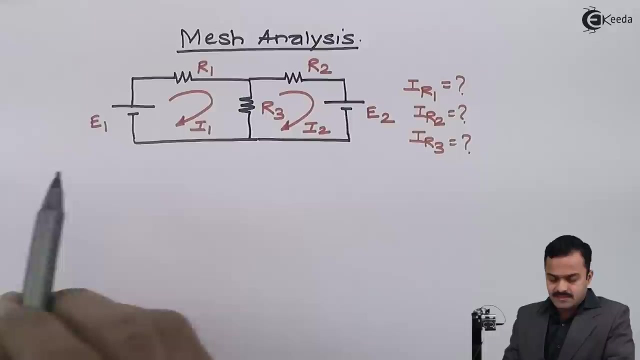 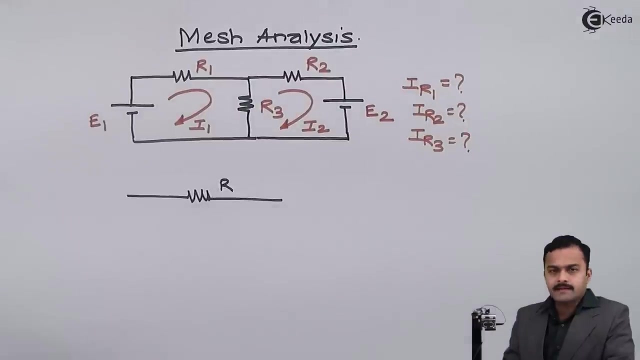 I will always consider clockwise direction for a loop current. Then, based on this direction of currents, I am going to mark voltage drops that got developed across all the resistances. So the concept is that whenever I am having a resistance like this and current I is flowing. 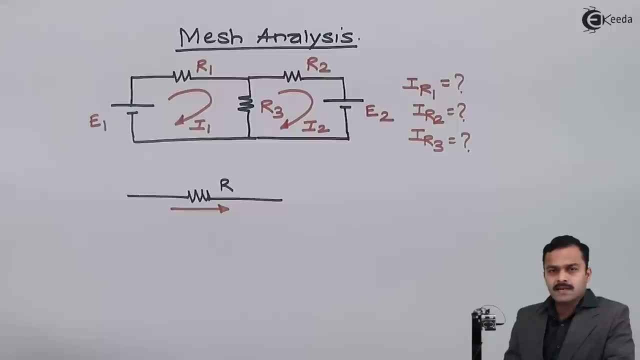 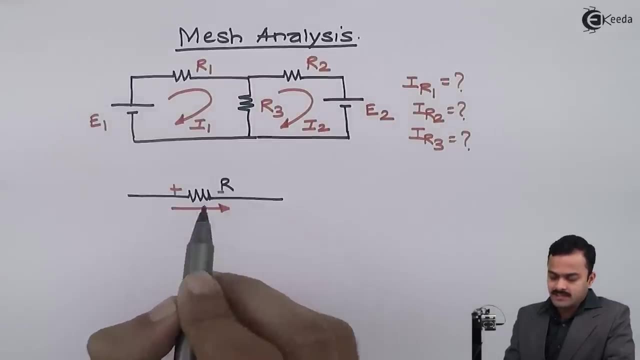 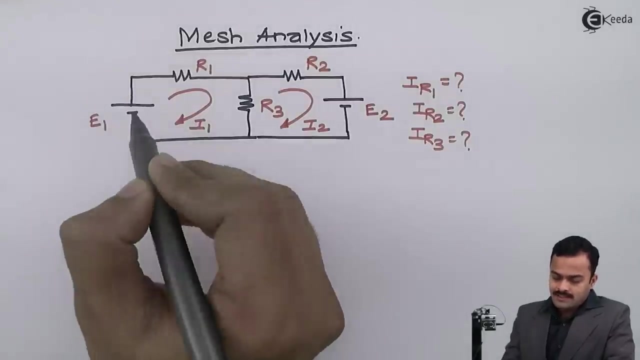 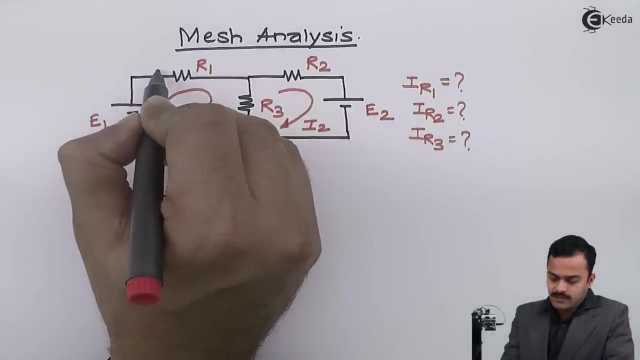 let's take in this direction. Then voltage drop developed across a resistance will be in the direction of current in this manner: plus minus, and that is considered as a drop. So let's mark all the voltage drops for these three resistances. So in the direction of current, I will get this polarity. 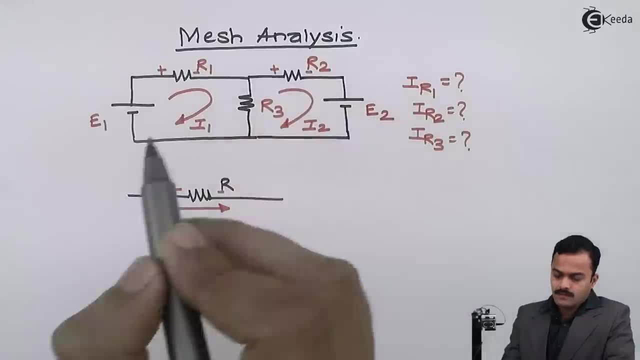 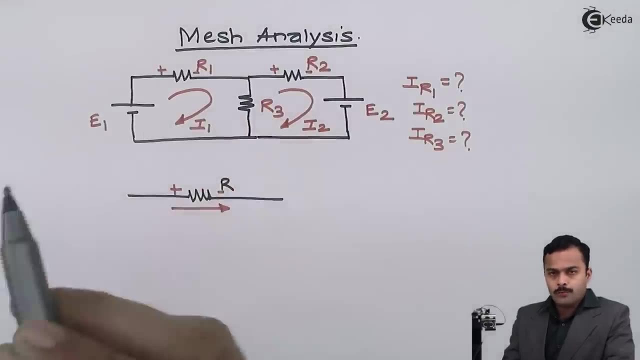 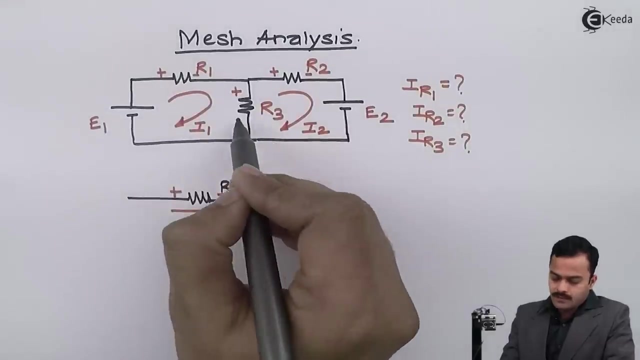 Now, R3 is a common resistance between loop 1 and 2. So obviously it will have two voltage drops. So as per I1,, it will have the voltage drop, this polarity, and as per the I2, it will have the voltage drop of the mentioned. 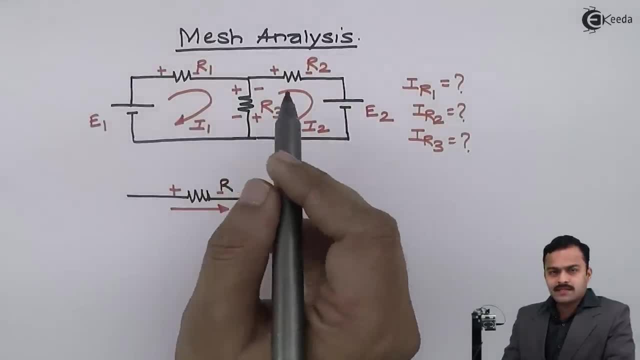 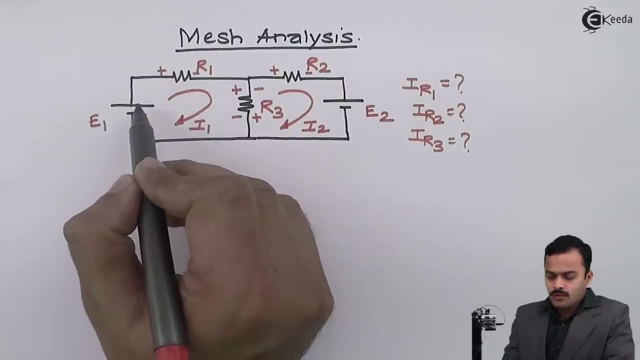 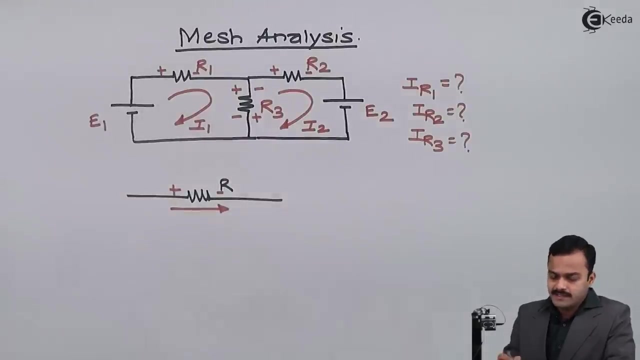 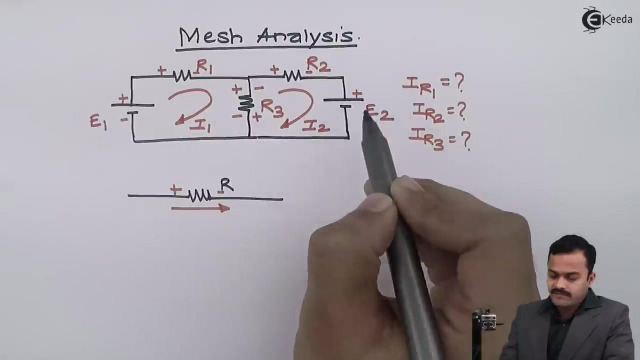 polarity. now, once you have done this, let's go back to the batteries. batteries, as we discussed earlier, the voltage or a potential of a battery does not depend upon direction of current. it will be fixed polarity and the polarity is longer arm plus, shorter arm minus. so same way I mark the polarities for E2. 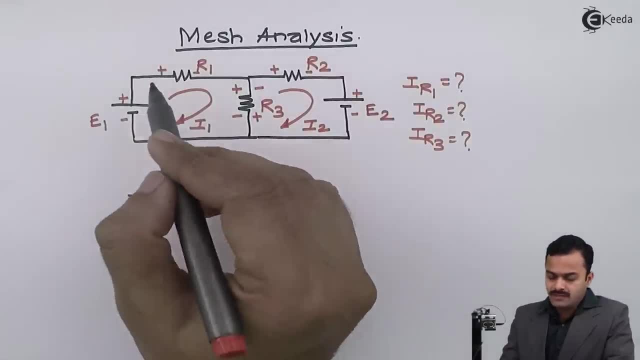 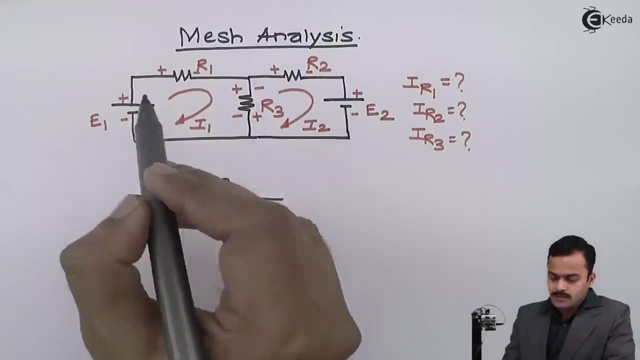 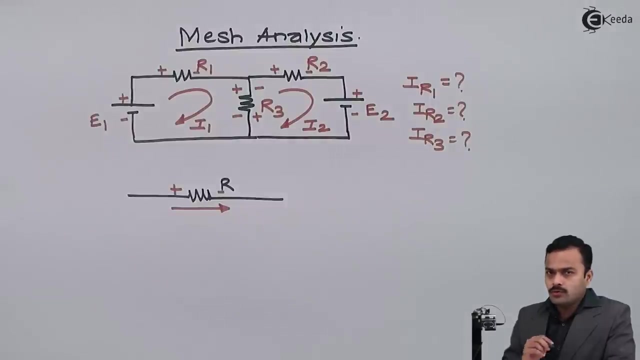 next, I need to trace a loop now, so I will trace loop in the direction of current only. that means in a clockwise direction for both the loops. so whenever I will trace a loop in the direction of current, I may come across two voltage drops or two voltages. 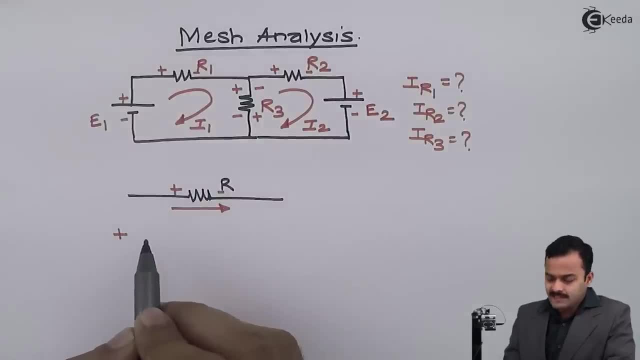 meaning I could have voltage changing from plus to minus or I could have voltage changing from minus to plus. if in the direction of a current voltage is getting developed like this- plus minus- then I will consider that as voltage drop and I will consider negative value for that while analyzing. 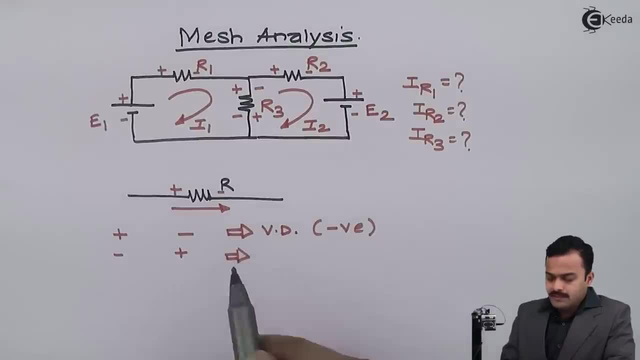 similarly, if in the direction of current voltage is changing from minus to plus, I will consider that as voltage rise and analysis purpose. I will take that as positive. now, keeping this in mind, I may write: let's apply KVL to a loop loop one. so I will apply KVL like this. so I'll start from this point and 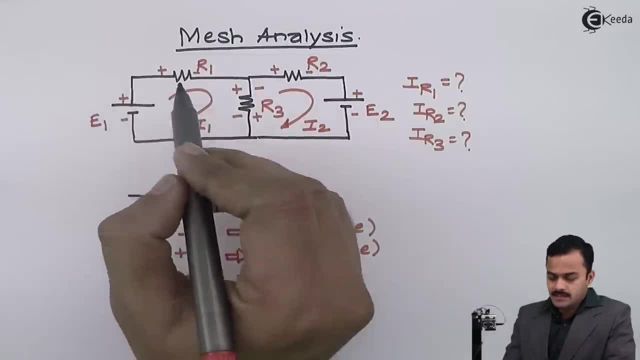 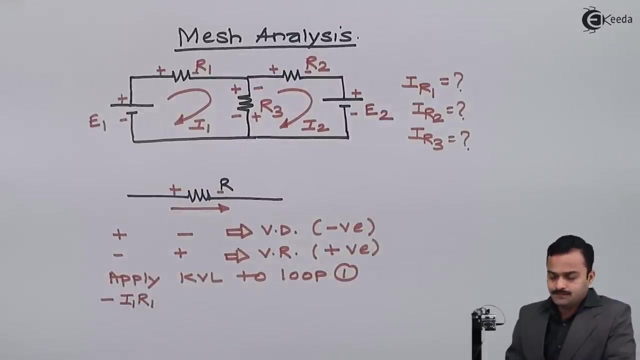 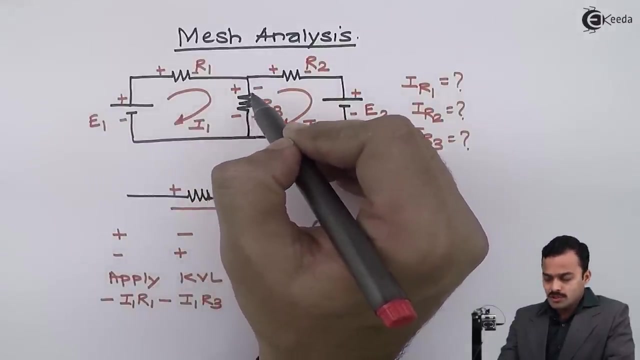 we'll come back to the same point after tracing these many elements. so plus, minus. plus minus is a voltage drop, so it is minus and voltage developed across a resistance will be current flowing through it, multiplied by resistance value. same way here, plus minus. so minus, minus, I1, R3, but in the direction of this current. I have one more voltage drop. 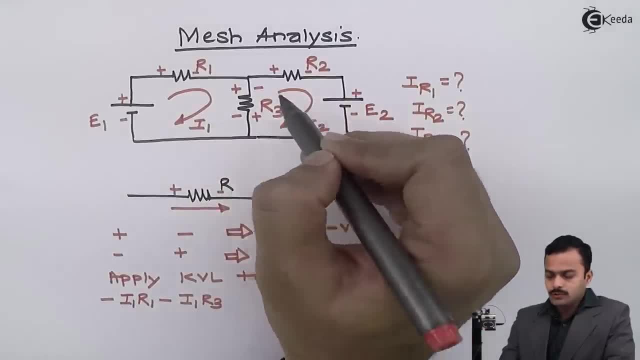 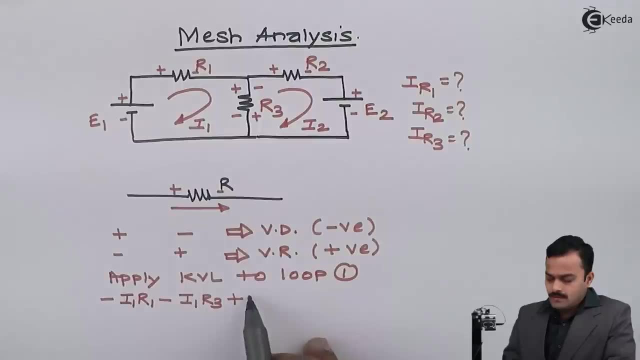 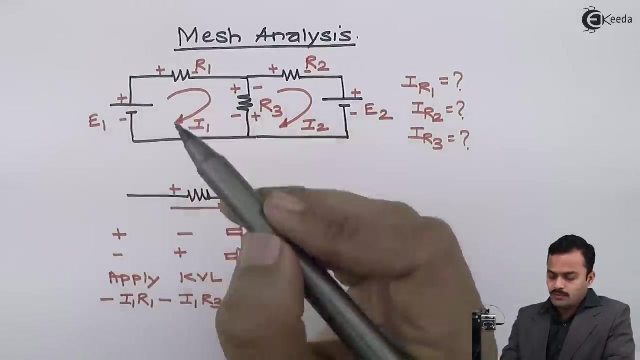 minus plus and that is developed because of the I2. so minus plus is voltage rise, so it's plus and it is developed because of I2, so it's I2 R3. and the third element is minus plus a potential difference of a battery. minus plus means it's a voltage right, so it's a plus constant. 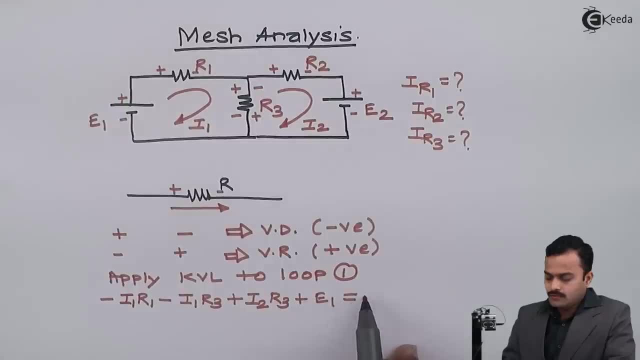 value E1 equal to zero. now I will simplify. I will club all I1 together so I will get like this: I will take this constant on another side of equation minus E1, equation number 1. similarly, I can apply KVL2, loop 2.. So loop 2. I will start from this point and we'll come back to the same point. 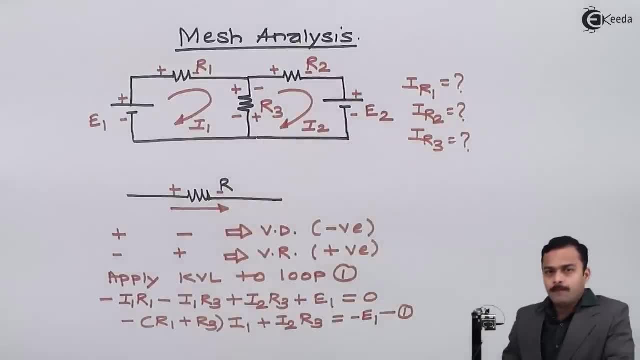 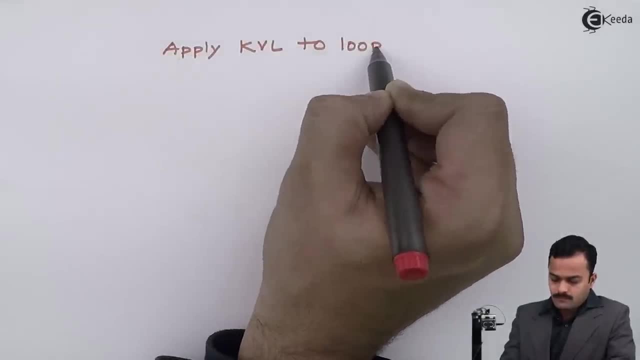 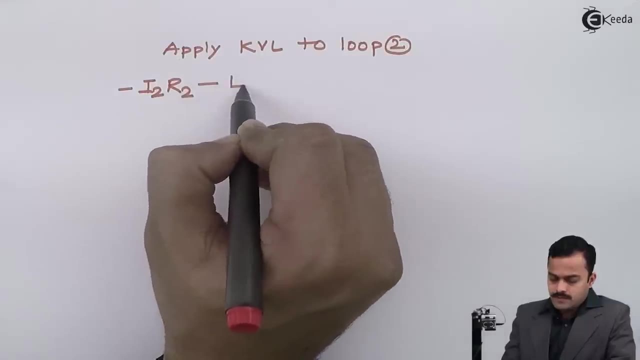 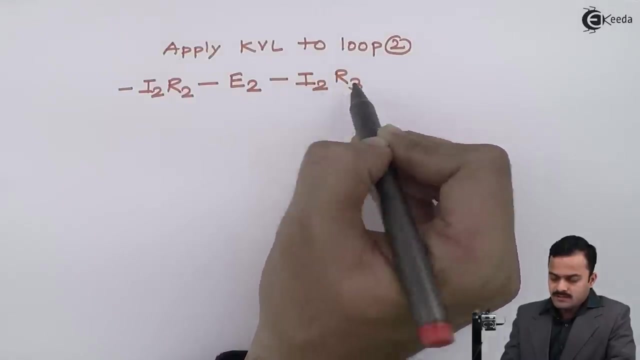 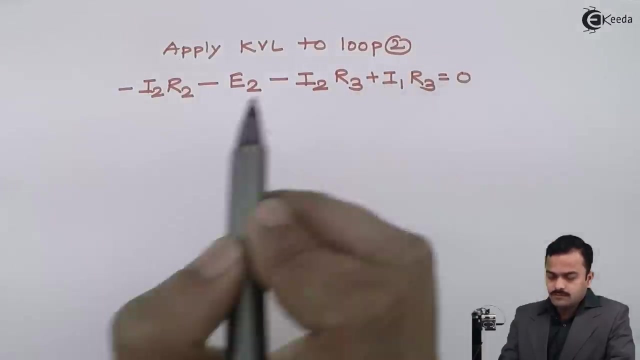 after tracing these many elements, along with the polarities of a voltage drop. So let's apply KVL2, loop 2.. So I will get minus I2 R2, minus E2, minus I2 R3, plus I1 R3 equal to 0.. Let me go back. 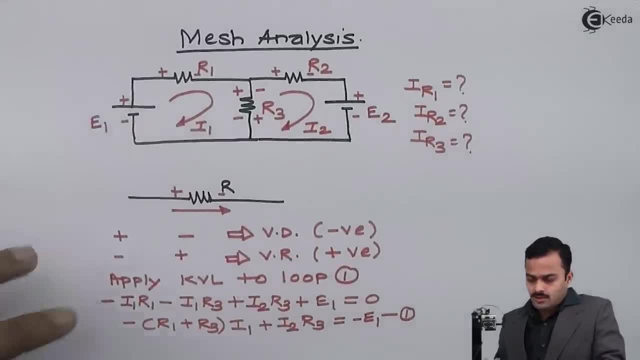 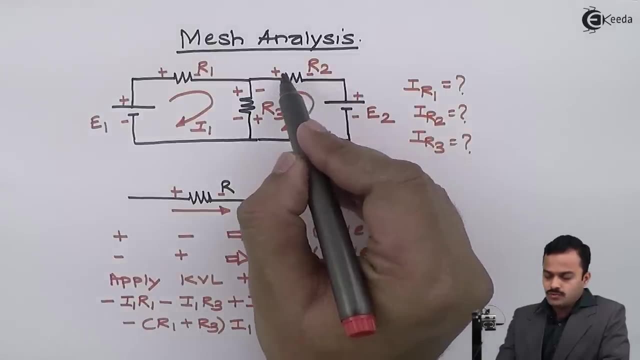 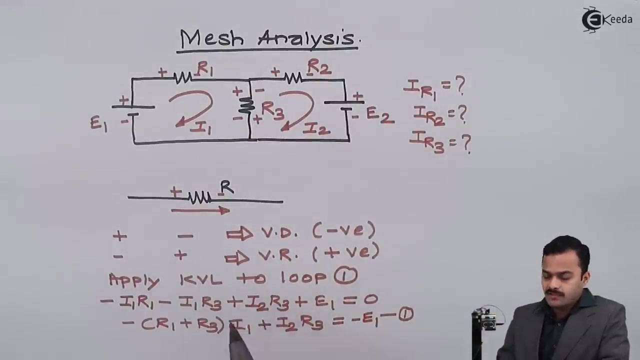 to a circuit once again. So I am considering this loop starting from this point and coming back to the same point. Plus, minus is a voltage drop, So minus I2 R2. plus minus is again a voltage drop, but this is a potential difference of a battery, So I will take that as it is minus E2.. Here again, two drops are. 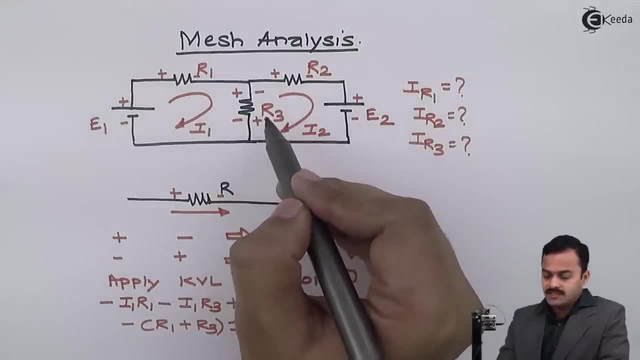 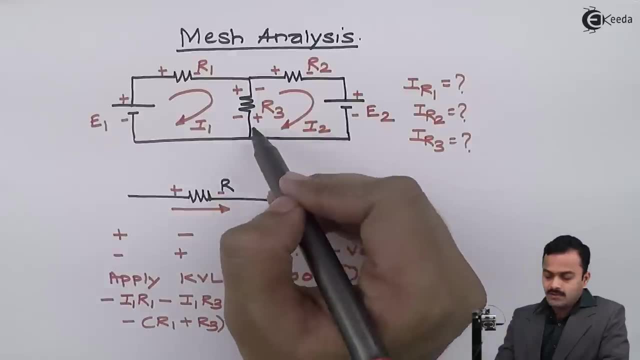 there. One is because of the I2.. So in the direction of I2 it is plus minus voltage drop and that is because of I2.. So minus I2, R3.. And in the direction of I2, one more drop is there: Minus plus. Minus plus is voltage right. 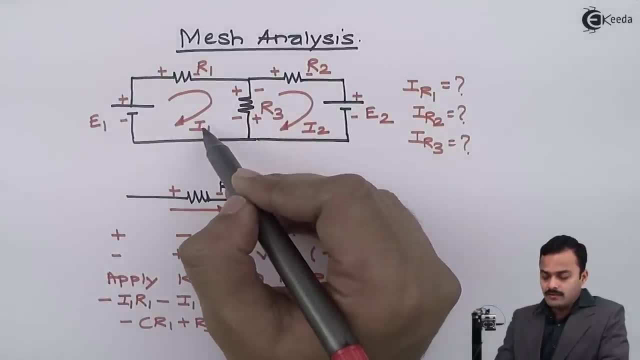 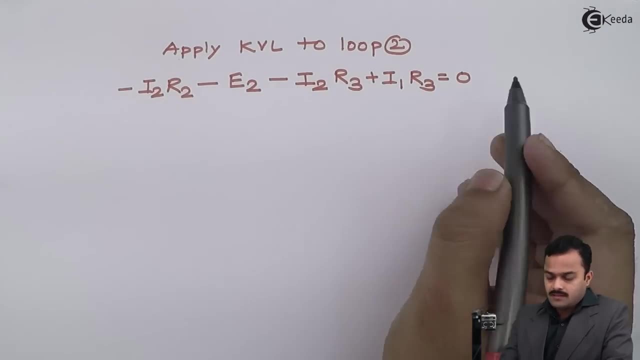 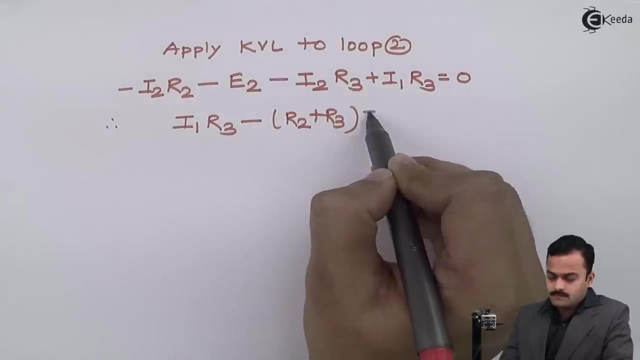 So I will take that as positive and that is because of I1.. So I1 R3. So that I will get finally this equation And after simplifying this, that mean I will rearrange the term, I will get this equation number 2.. 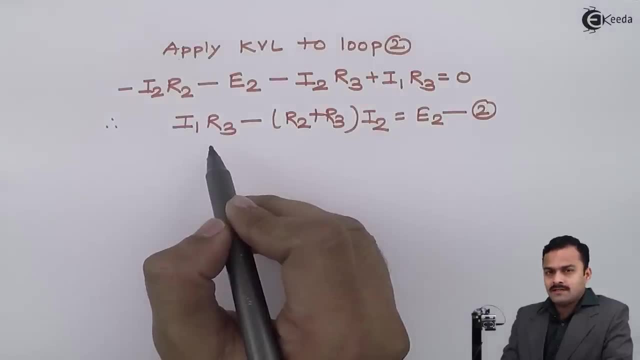 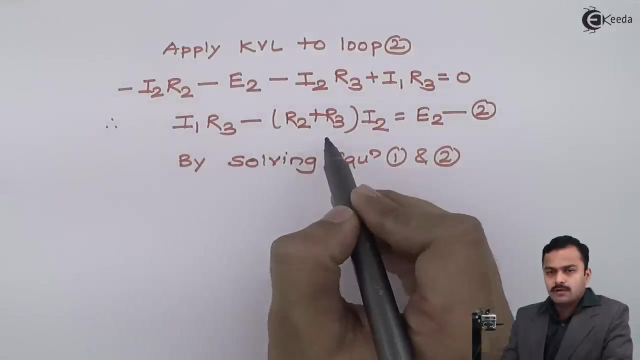 is to find out value of current flowing through all the resistances. for that I should know all loop currents. so by solving equation 1 and 2, obviously, whenever we solve numerical we will have the value instead of R 1, R 2, R 3 e 1 and. 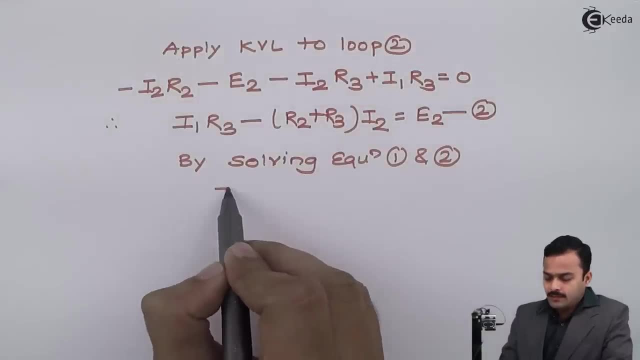 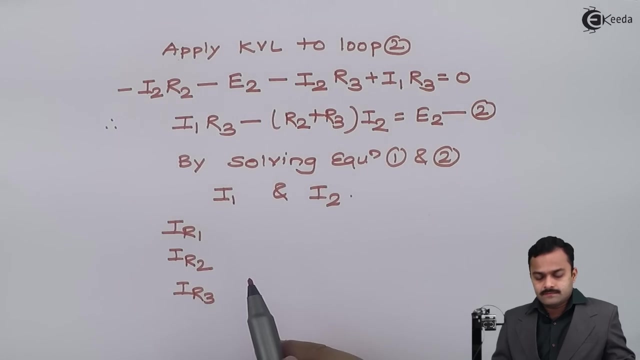 e 2, so obviously you will have a number and then you can get a value of I 1 and value of I 2. now, using these two loop currents, I am supposed to get the value of IR 1, IR 2 and IR 3. so let's go back to the circuit once again. so if I see, 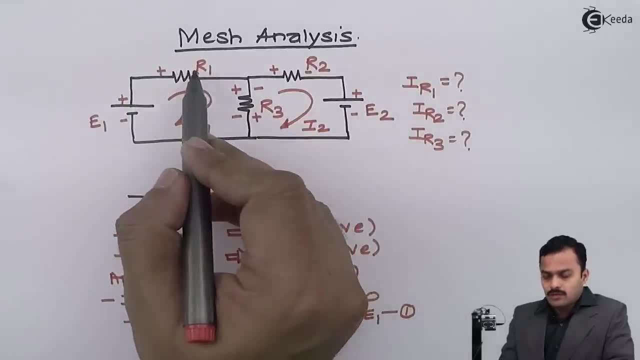 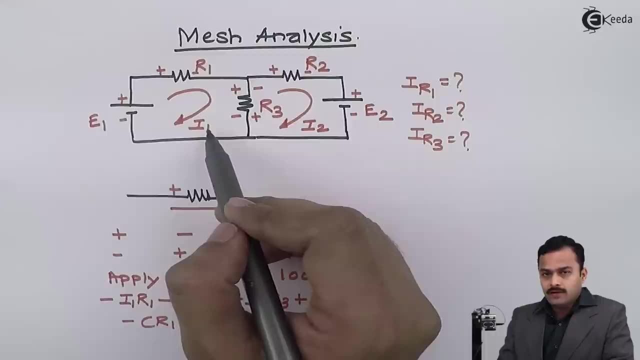 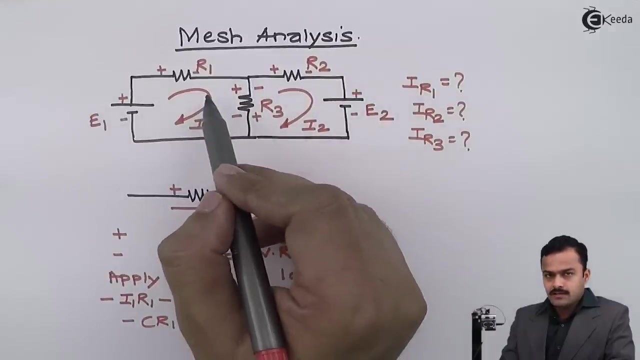 properly. the current flowing through the R 1 is nothing but I 1 only. current flowing through the R 2 is I 2 only. but current flowing through the R 3 it may be I 1 and I 2, but not necessarily that will be I 1 plus I 2. it all depends upon the direction of current.